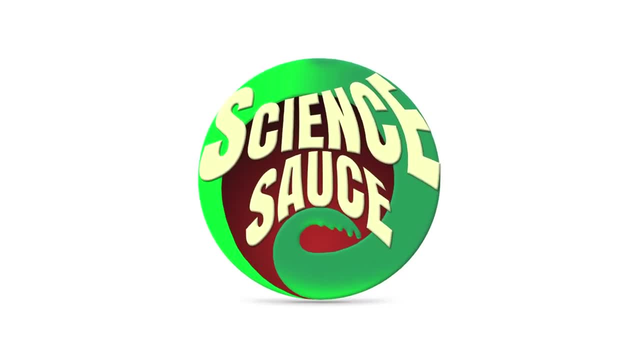 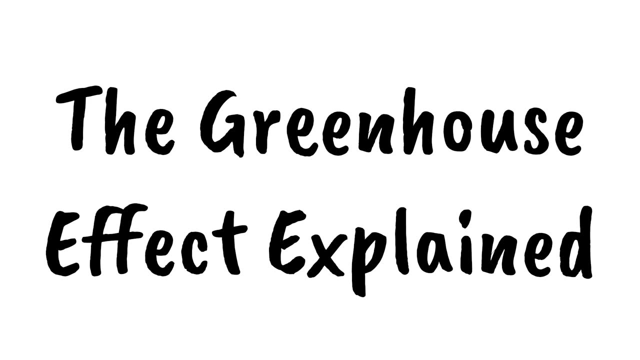 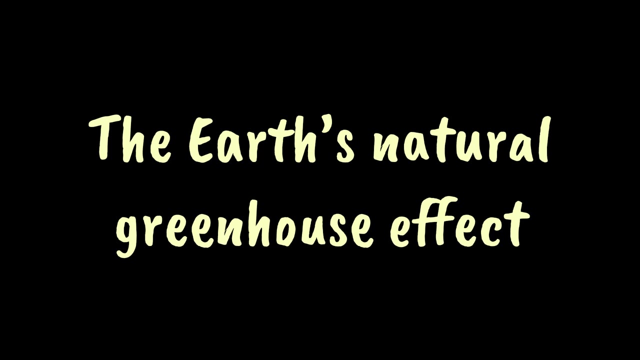 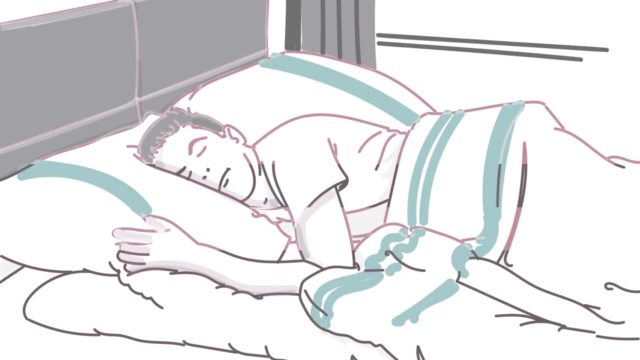 Before we start, I need to be clear that this video is about the Earth's natural greenhouse effect. This is not a discussion about global warming or climate change, but I will make the link to climate change briefly at the end. The greenhouse effect can be thought of a bit like: 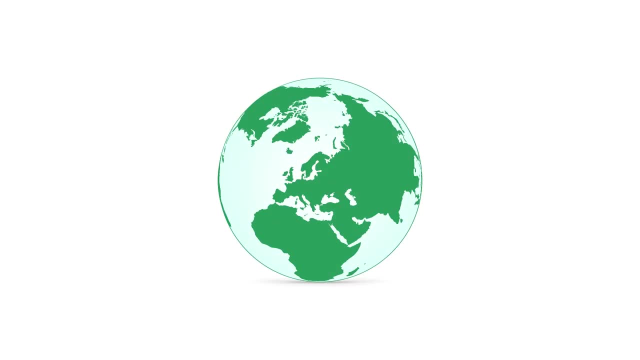 the blanket you cover yourself with at night to keep warm. Our planet has an atmosphere around it containing certain gases that trap heat energy. helping to keep the planet warm And no matter what anyone tells you, the greenhouse effect is a very good thing. 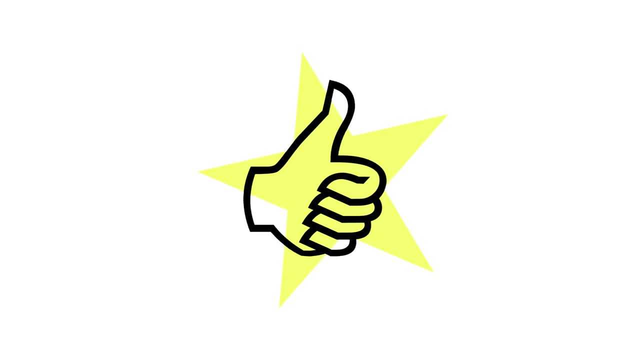 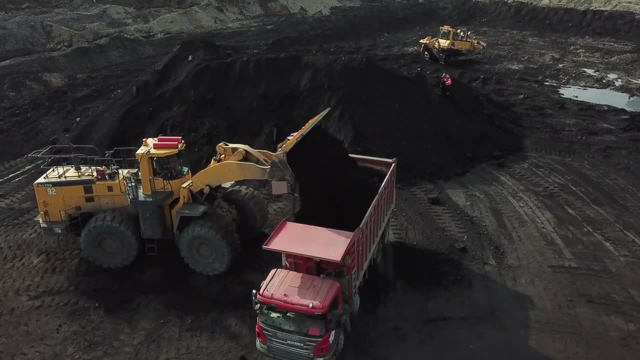 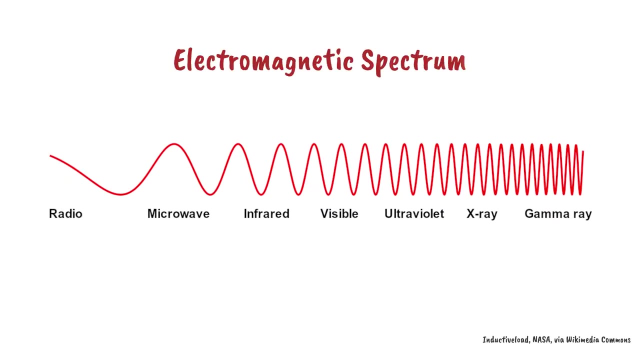 No scientist would ever challenge that statement. The greenhouse effect is an entirely natural process. It was taking place long before the first lump of coal was ever burnt or the first cow let one rip. The explanation starts with energy waves presented here on the electromagnetic spectrum. 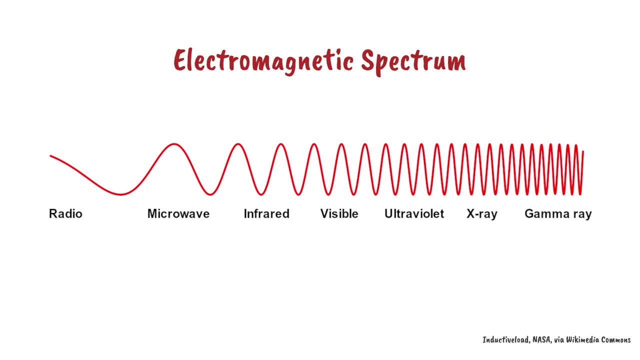 Radio waves, light, x-rays- they're all basically the same thing. We often think of them as travelling in waves, and the thing that makes them different from each other is the length of that wave. To understand the greenhouse effect, we're interested in infrared waves. 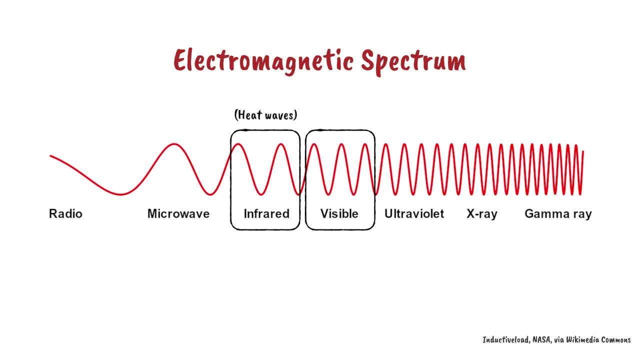 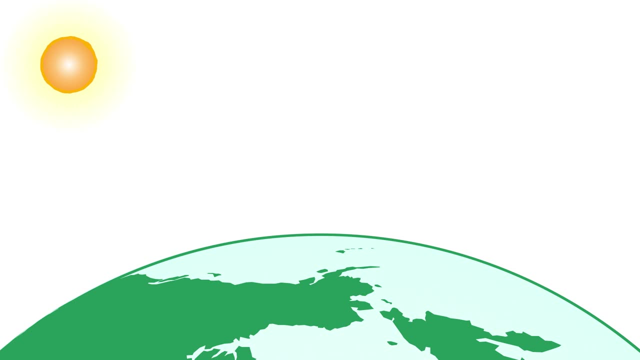 a fancy term for heat waves as well as visible light. Notice that infrared waves have a longer wavelength than light waves. That's an important detail. As you probably know, we get our energy from the sun. The energy from the sun reaching our planet is mostly in the form. 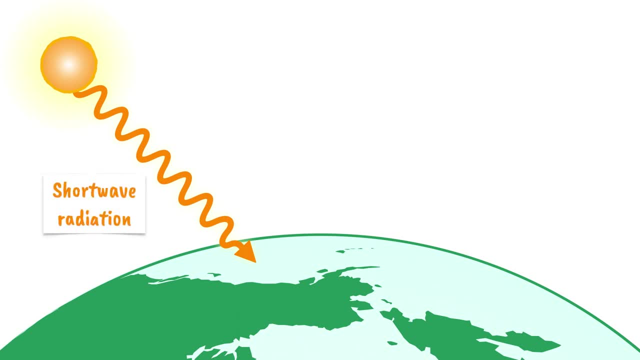 of light energy. We'll call this shortwave radiation to keep things simple. Some of that energy is absorbed by the planet's surface, causing an increase in temperature. Energy that has been absorbed and warmed an object can then be released, But it isn't released. 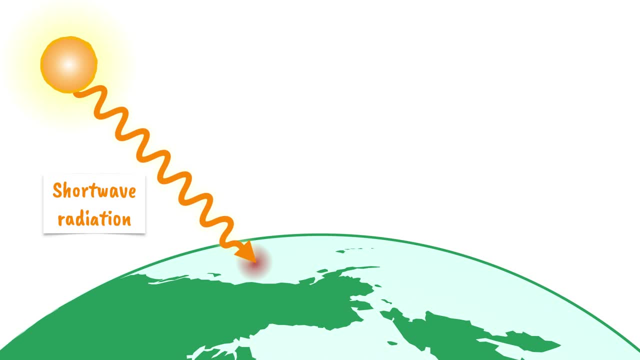 as light energy. The energy is released or re-emitted, to use the correct term- as infrared waves, Heat in other words. Remember that these heat waves have a longer wavelength than the light waves that first reached the surface. From here on in, we'll call these infrared waves longwave. 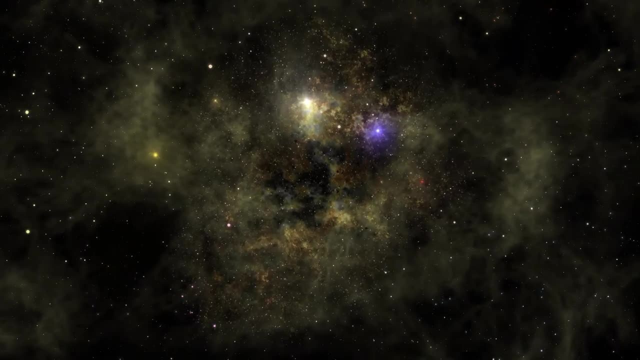 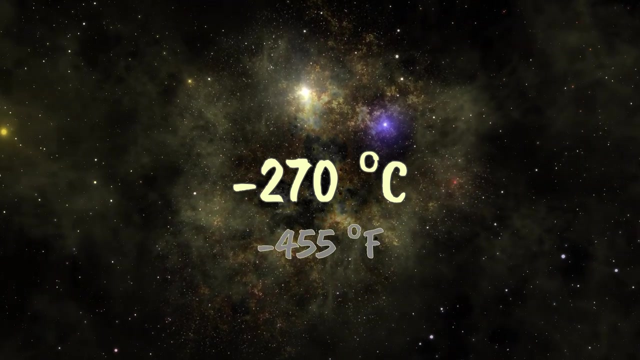 radiation. Next, let's look at space. Space is cold. Its baseline temperature is about minus 270 degrees Celsius. Very cold indeed, Far too cold for life to exist. Fortunately, since our planet orbits close to the universe, our life is not as cold as it was before. 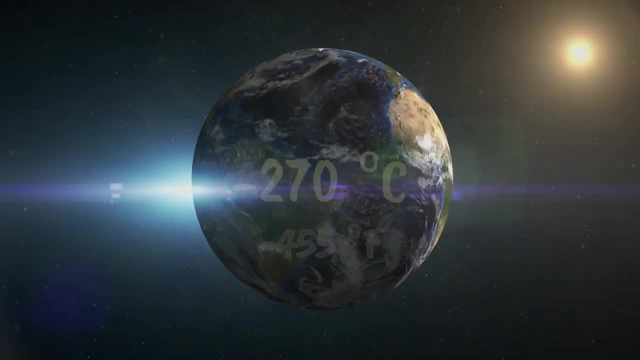 In fact, very slightly colder than the previous temperature right above our head. That's how the first wave of the earth is unable to differentiate the temperature. The first wave is clearly less cold as compared to the second wave of the earth, far too cold for life to exist, Fortunately, since our planet orbits close to the sun. 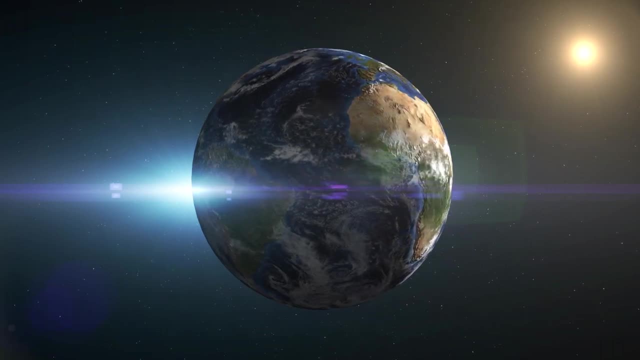 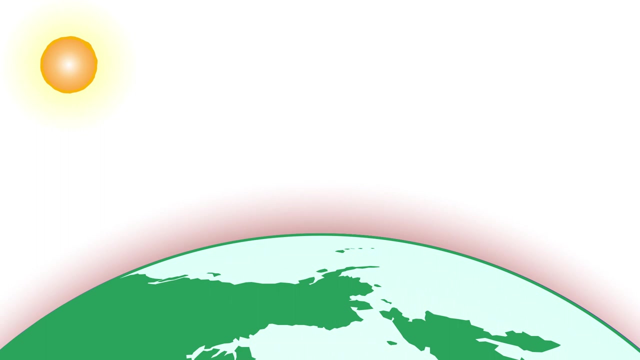 close in astronomical terms. that is, we are kept well above that temperature. However, if the earth were to absorb and re-emit energy the way I've already described and all of that long wave radiation is allowed to leave the earth system, the average temperature of the earth would be around minus 18 degrees celsius. 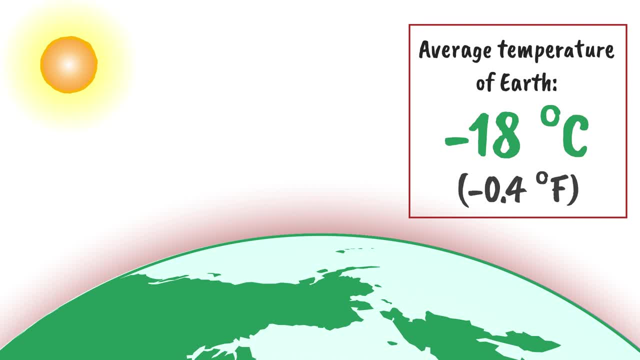 That's better than the minus 270 of space, but still fairly cold. We know the earth isn't really that cold. so what are we missing? Enter the greenhouse effect. Fortunately for us, specific gases in our atmosphere, gases such as carbon dioxide. 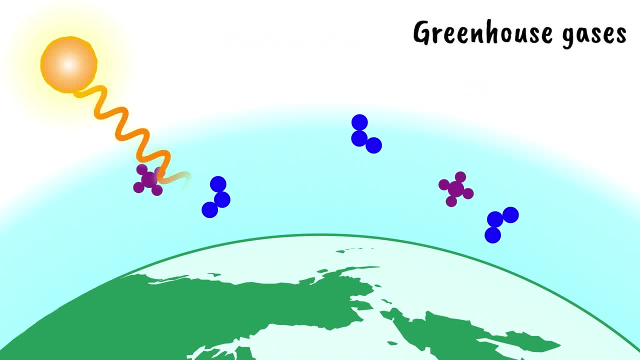 methane and others, all known as greenhouse gases, are able to absorb and re-emit the long wave radiation coming from the surface of the earth. Now remember: short wave radiation reaches us from the sun, but long wave radiation is radiated from the surface. 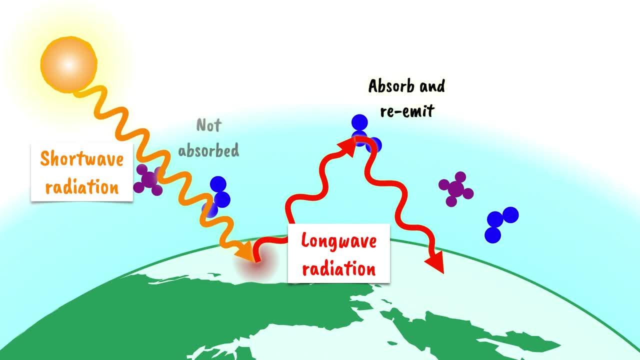 These greenhouse gases are not able to absorb short wave radiation reaching the earth. Consequently, they let the sun's energy in, but then trap some of it as it tries to leave. This trapping of heat energy obviously raises the temperature in the atmosphere, earth's surface and its oceans. 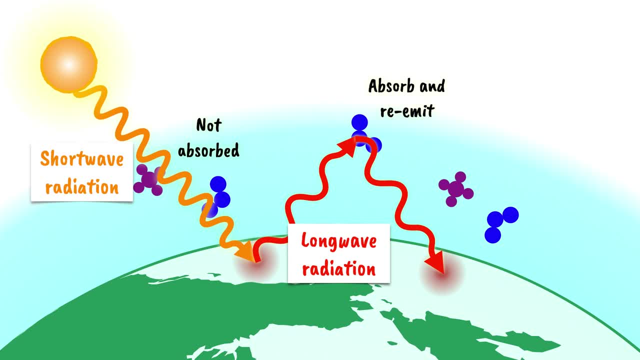 So, basically, our atmosphere traps some of the heat energy that we're getting from the sun and then traps some of it as it tries to leave. This is because it traps the sun's energy in the atmosphere and traps some of the heat energy in the earth system. 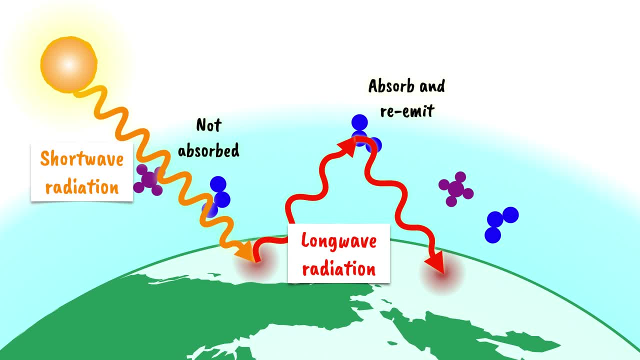 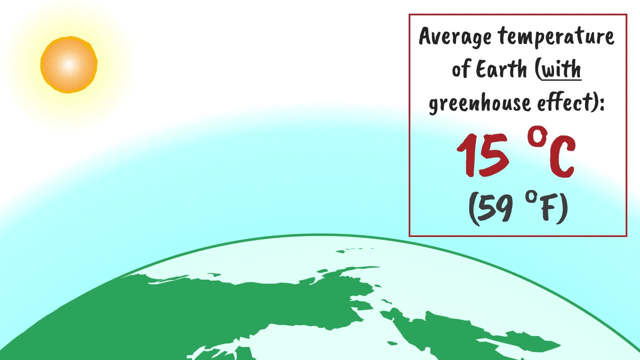 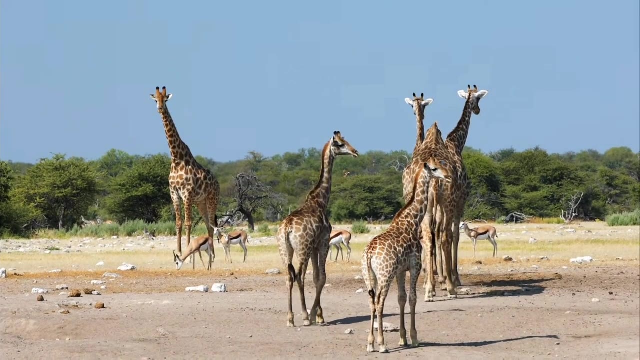 keeping it that bit more warm. As a result of earth's natural greenhouse effect, the average temperature on our planet is about 15 degrees celsius- 33 degrees warmer than it would be without any greenhouse effect. It's because of this natural greenhouse effect that our planet can sustain life. 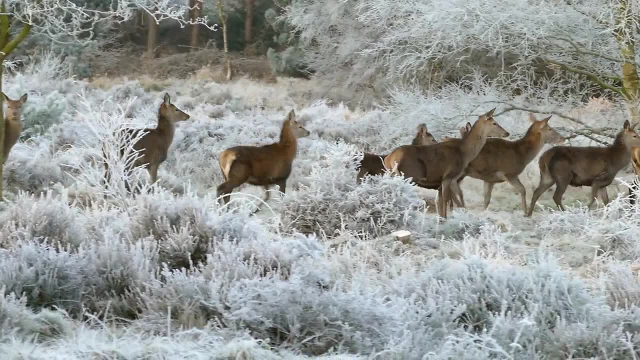 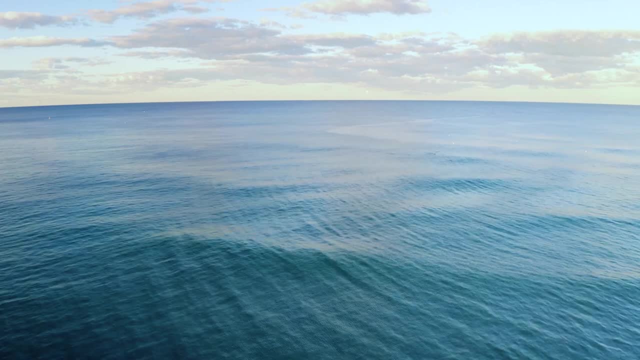 While the earth obviously has hot and cold regions, the average temperature of around 15 degrees celsius Celsius is warm enough that water exists in liquid form over much of the planet Without a greenhouse effect. the low temperature of minus 18 degrees Celsius would result in most. 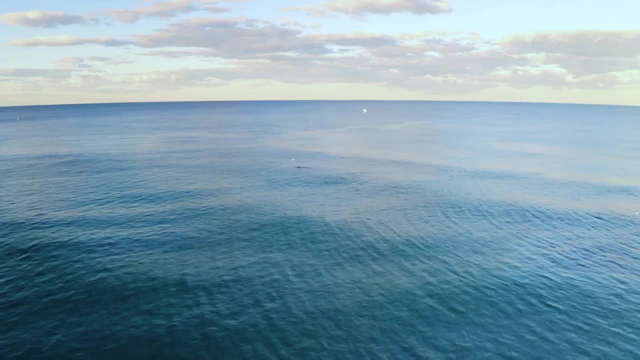 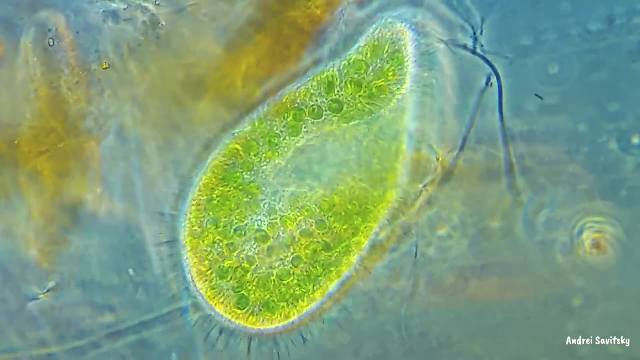 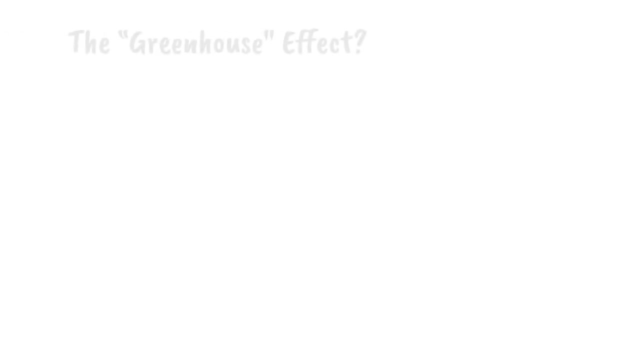 of Earth's water being locked up as solid ice. Without liquid water as a medium for chemical reactions in cells to take place, life as we know it simply couldn't exist. Oh, and you may wonder why it's called the greenhouse effect. Well, in case you didn't,